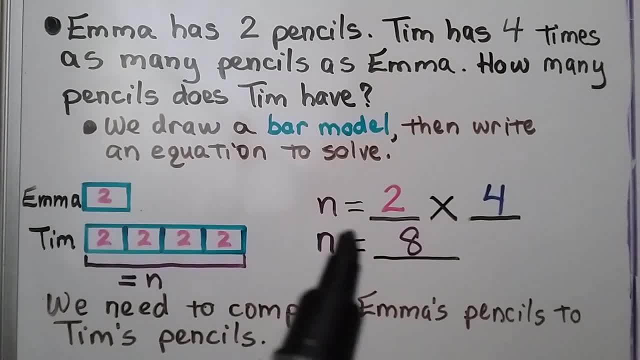 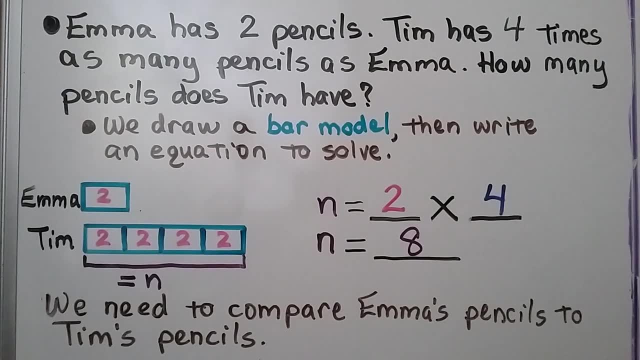 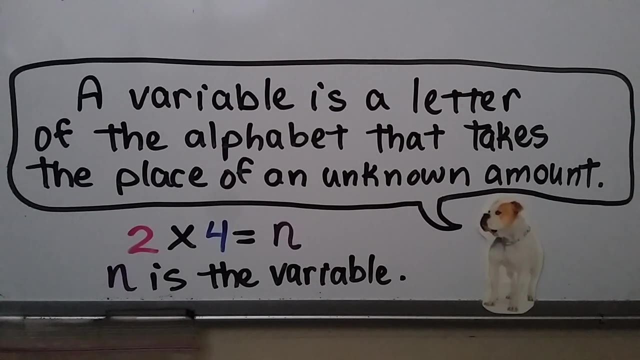 Tim's total is equal to n, and n is equal to 2 times 4,, which is equal to 8.. We need to compare Emma's pencils to Tim's pencils. A variable is a number. It's a letter of the alphabet that takes the place of an unknown amount. 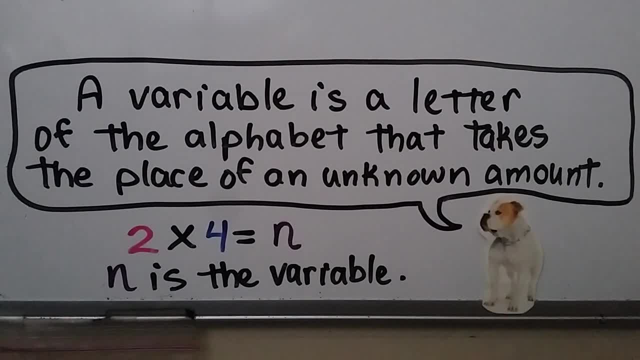 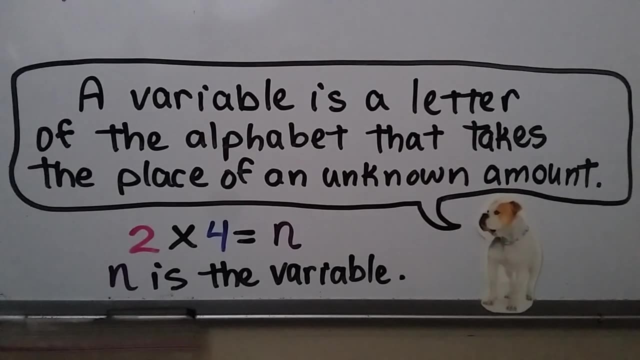 So instead of using a blank space or an empty box, we use a variable. We use it in algebra, So we would have: 2 times 4 is equal to n. That's the unknown amount, n is the variable, And it could be pretty much any letter of the alphabet, except we don't use an o because it could get confused with a zero. 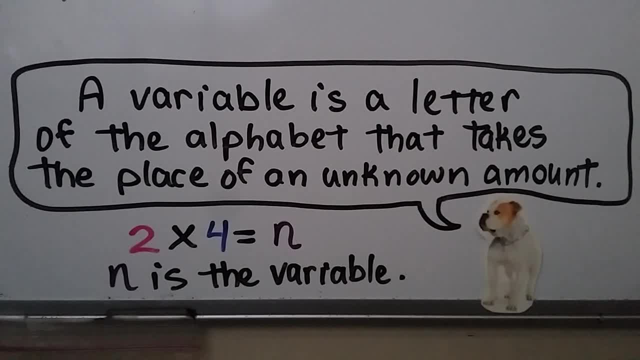 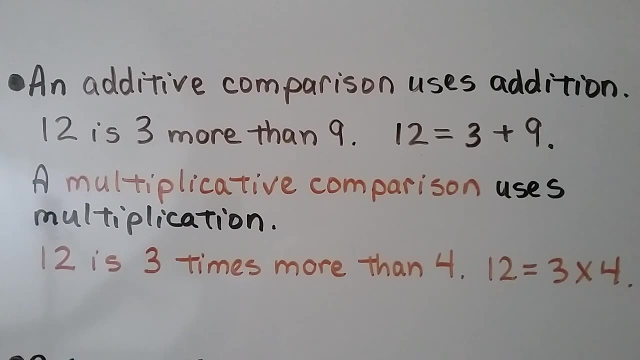 And a lowercase l could get confused with a, 1.. So you're usually going to see n or x or b or c, p, q, r are used a lot. Those are all variables. An additive comparison uses addition 12 is 3 more than 9.. 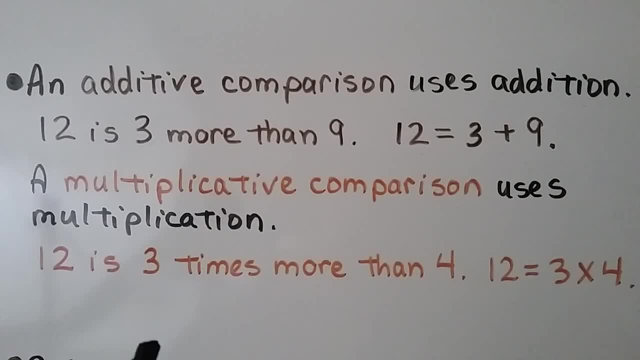 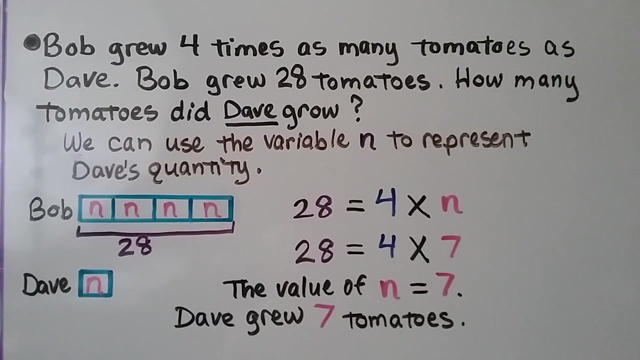 12 is equal to 3 plus 9.. A multiplicative comparison uses multiplication. 12 is 3 times more than 4.. 12 is equal to 3 times 4.. Bob grew 4 times as many tomatoes as Dave. 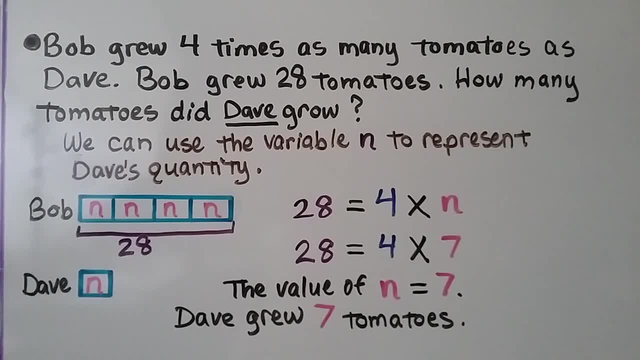 Bob grew 28 tomatoes. So how many tomatoes did Dave grow? We can use the variable n to represent Dave's quantity. That's what we're trying to find. How many tomatoes did Dave grow? So Bob grew 28,, and it was 4 times as many as Dave's. 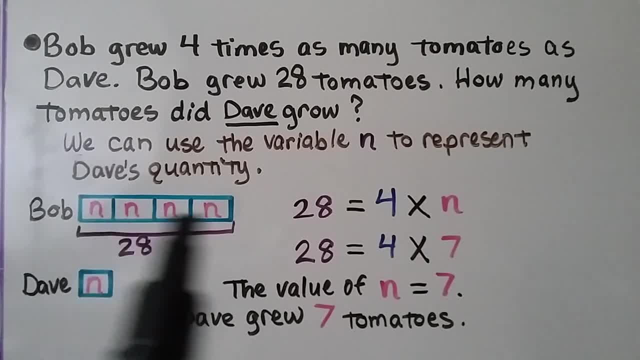 So Dave would be 1n and Bob's would be 4n, because it's 4 times 28 is equal to 4 times n. Well, if you know your multiplication facts, you know 4 times 7 is equal to 28.. 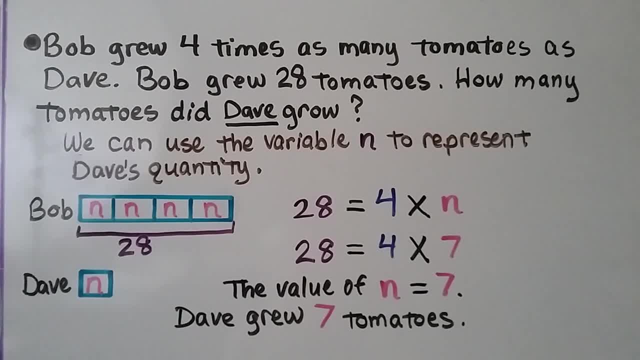 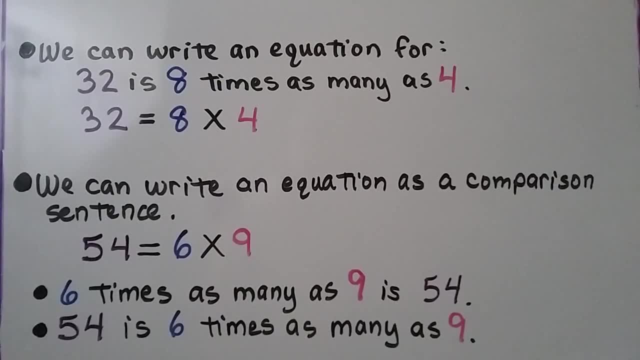 So the value of n is equal to 7.. Dave grew 7 tomatoes. We can write an equation for: 32 is 8 times as many as 4.. 32,- our equal sign is the- is 8 times as many as 4.. 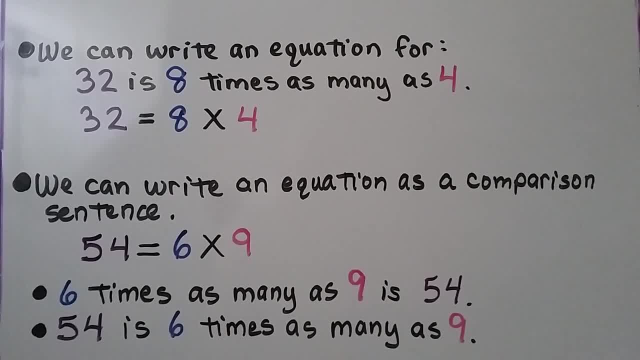 And we can write an equation as a comparison sentence: 54 equals 6 times 9.. We can write 6 times as many as 9 is equal to 54.. We can also write: 54 is 6 times as many as 9.. 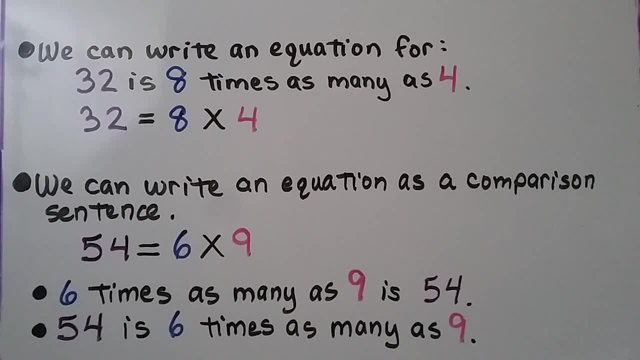 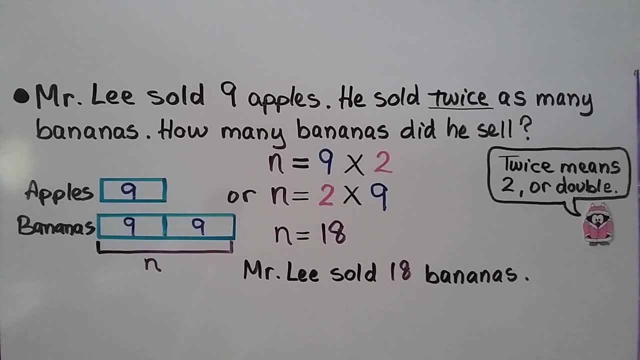 It all is the same thing. They have the same meaning. Mr Lee sold 9 apples. He sold twice as many bananas. How many bananas did he sell? So the word twice means 2, or double. So that means he sold 2 times as many as he sold apples. 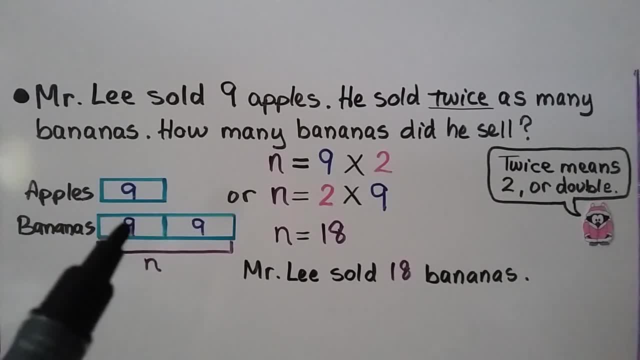 Here's his apples He sold 9.. Bananas is 2 times that, so we have 2 of them And that's going to equal our unknown amount. our n, our variable n, is equal to 9 times 2, or we could write it as 2 times 9,, couldn't we? 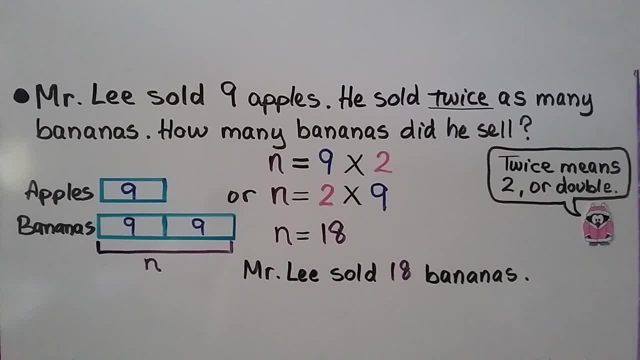 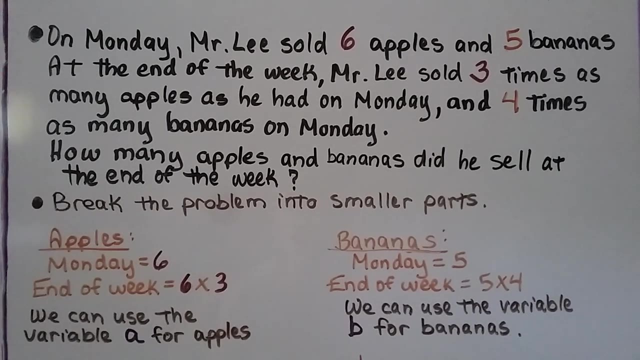 Because the commutative property states that we can multiply two factors in any order and get the same product. n is equal to 18.. So we know Mr Lee sold 18 bananas. On Monday, Mr Lee sold 6 apples and 5 bananas. 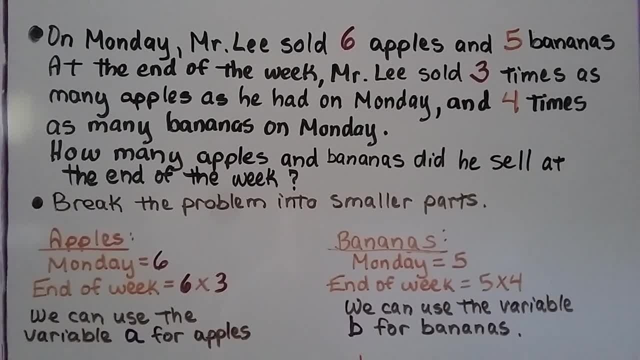 At the end of the week, Mr Lee sold 3 times as many apples as he had on Monday and 4 times as many bananas on Monday. How many apples and bananas did he sell by the end of the week? Well, he sold 6 apples and at the end of the week, sold 3 times as many as that: 6.. 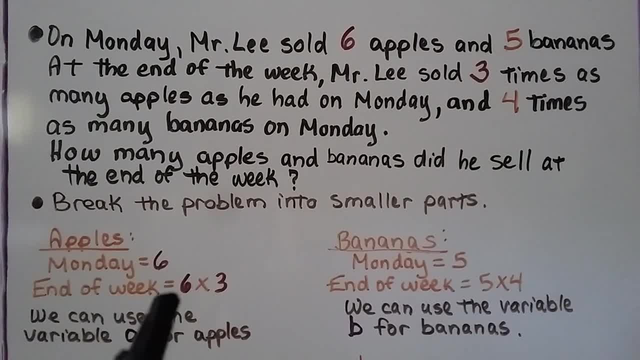 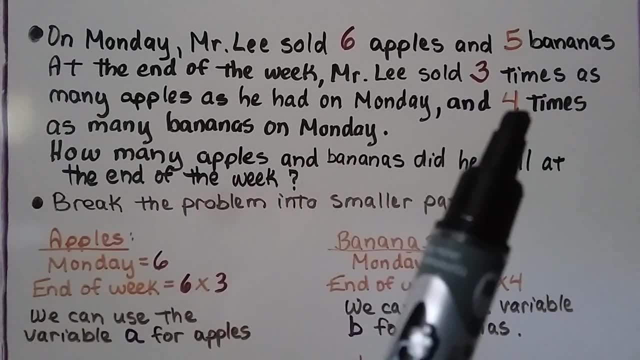 So Monday was 6.. By the end of the week he had sold 6 times 3.. For the bananas on Monday he sold 5, and at the end of the week he sold 4 times as many as that. 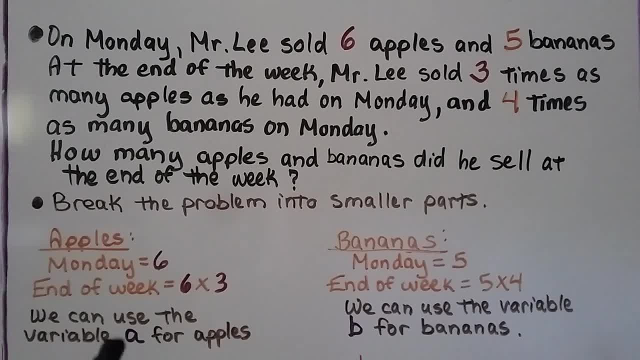 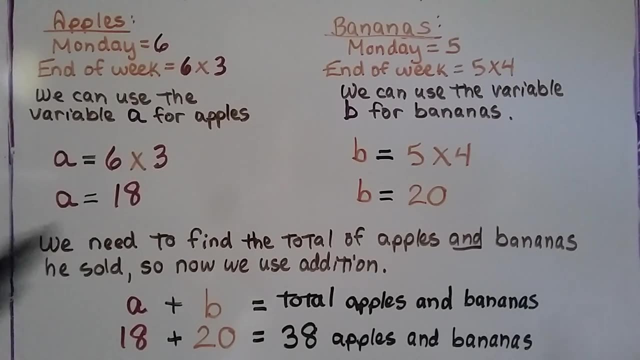 So that's 5 times 4.. And we can use a variable, a for apples and b for bananas, So a would be the 6 times 3, that's the apples. So apples is equal to 3.. So apples is equal to 18.. 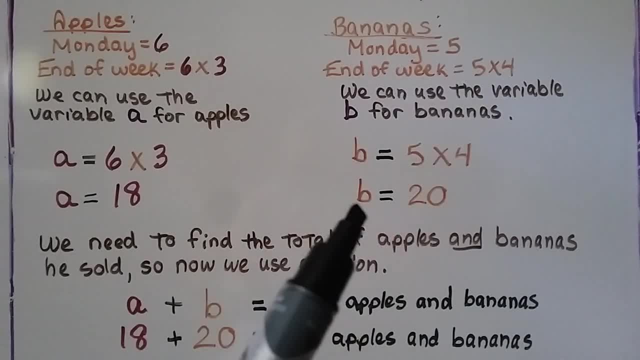 And b is 5 times 4,, which is equal to 20.. So b is equal to 20.. We need to find the total of apples and bananas he sold. Now we use addition. We need to add the a plus the b for the total apples and bananas. 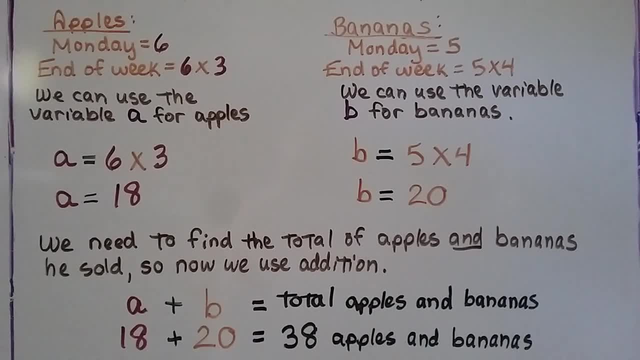 We add the 18 plus the 20. That's 38 apples and bananas that Mr Lee sold by the end of the week. We have three items in this menu. We're going to look at domestically delicious и chocolaty Ice cream. 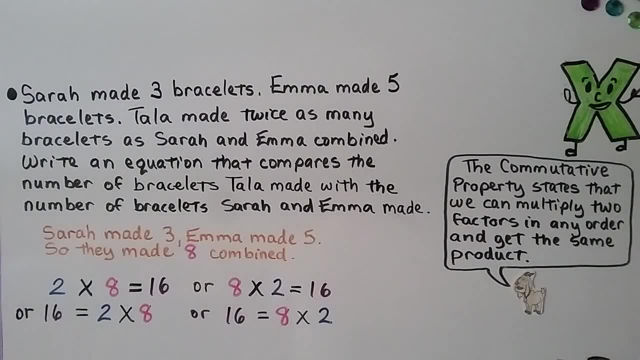 They're a trusted brand In Korea, they are dressed in Western style And you can sell them for 80 dollars, That's through January. 2 times 8,, that's equal to 16.. And because the commutative property states that we can multiply two factors in any order. 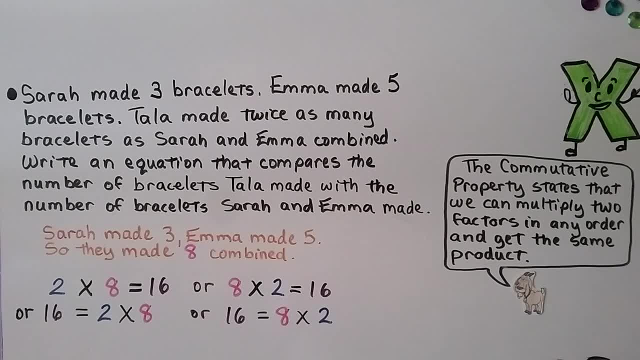 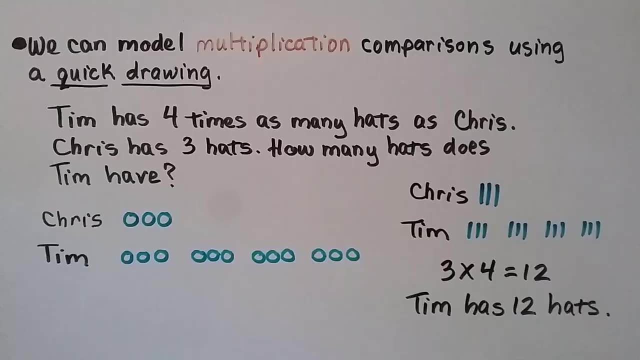 and get the same product. we can write: 8 times 2 is equal to 16.. We can even write it with the 16 in the front: equals 2 times 8, 16 equals 8 times 2. And it has the same meaning. 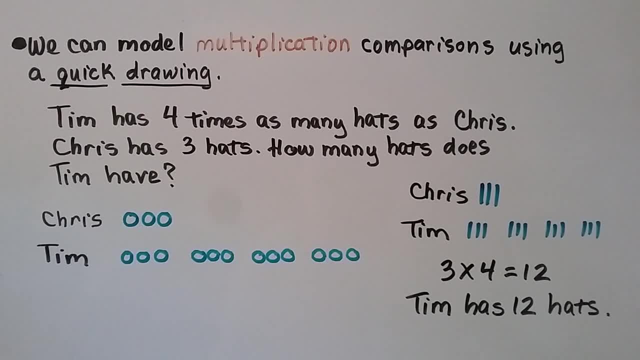 We can model multiplication comparisons using a quick drawing. Tim has 4 times as many hats as Chris. Chris has 3 hats. how many hats does Tim have? We know Chris has 3, so we can make 3 little circles. and if Tim has 4 times as many, we. 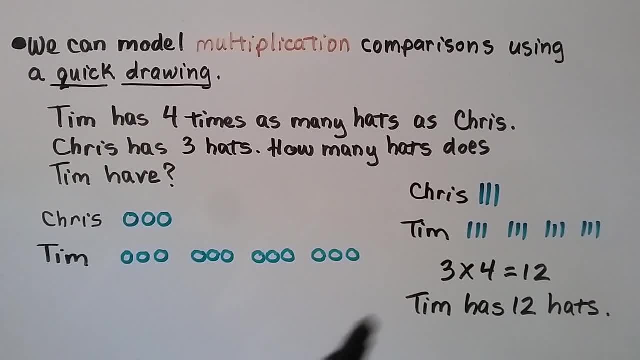 make 4 groups of 3.. We could even use tally marks. Chris has 3 hats. Tim has 4 times as many. we make 4 groups of 3.. And Three times four is equal to twelve. so we know Tim has twelve hats. 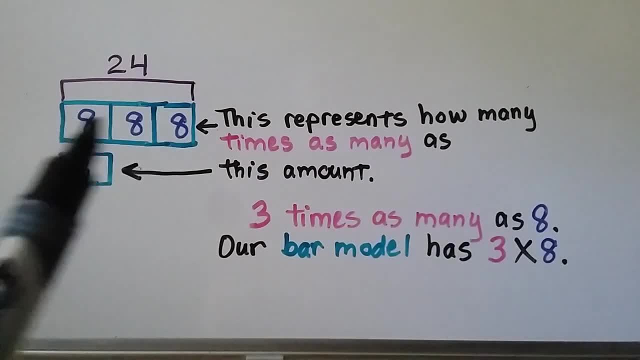 And remember, when you see a bar model, this represents how many times as many as this amount. So we have an amount eight. now we have three times as many, three times as many as eight. So our bar model has three times eight, which is equal to twenty-four, isn't it?